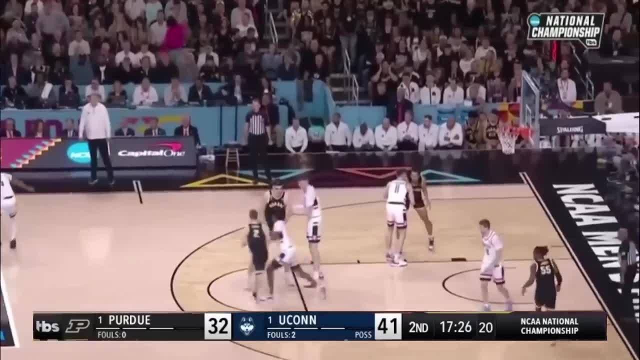 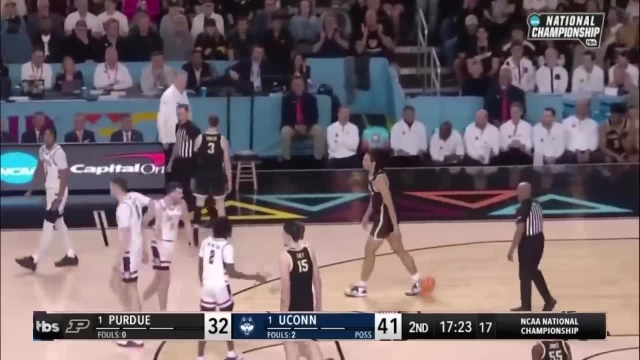 And it's bouncy castle on the inside- Almost a 10-second call. right there They got a foul. Oh no, it's going the other way. Kaufman rent, that is where you got to be concerned right now, if you're Purdue for tonight. 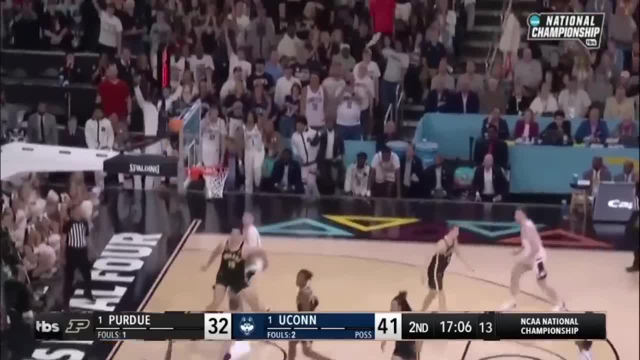 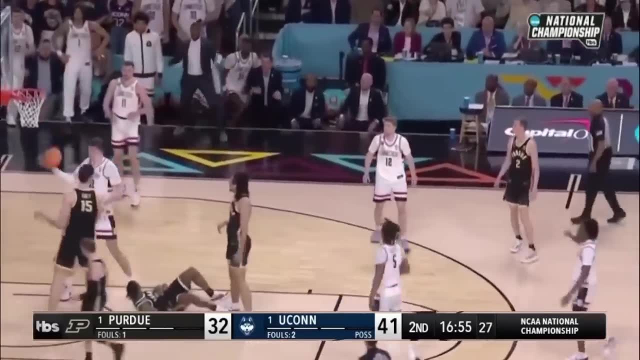 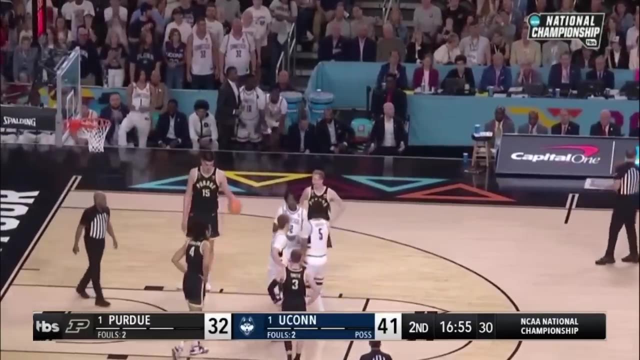 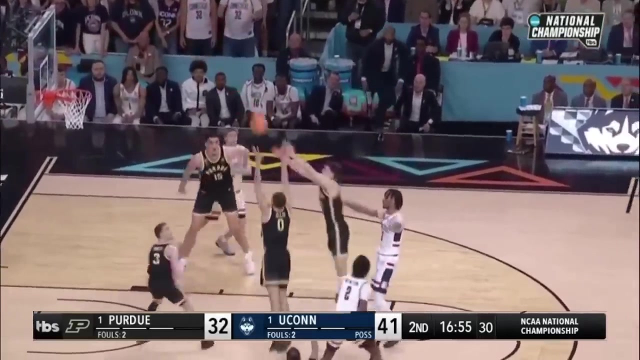 You need not guard anybody. Newton lets it fly. Rebound, happen remedy didn't track it down on for right now castle contact And it's a blocking foul on. are you gonna mention per diem again, right, And now Jones sits with those three fouls. we a must. the premise of the Yukon program is, with defensive rebounding, the 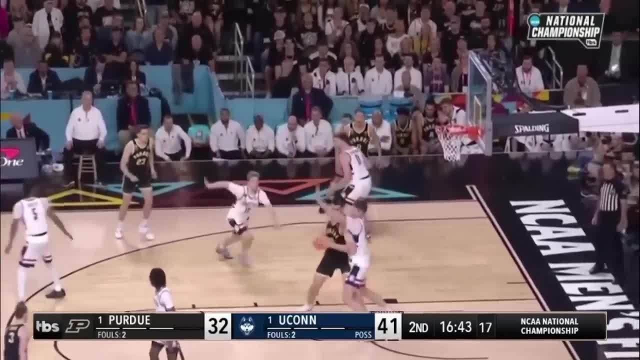 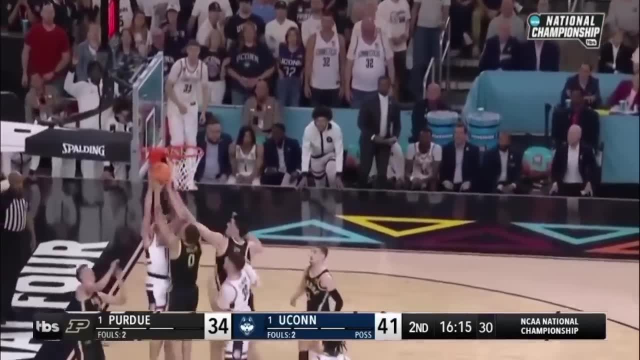 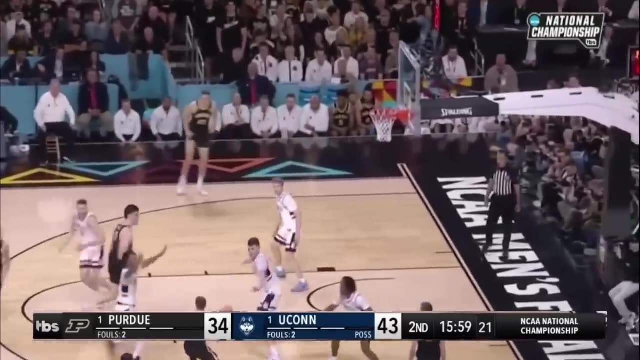 Opinion that it should have been offensive lawyer. feed it eating Mr. Through this crowd. Spencer doesn't go rebound, Castle is there, can't get it on the first clean up and he put it over eight, seven of nine. He's missed his last six shots. Hello, look at them, load up. 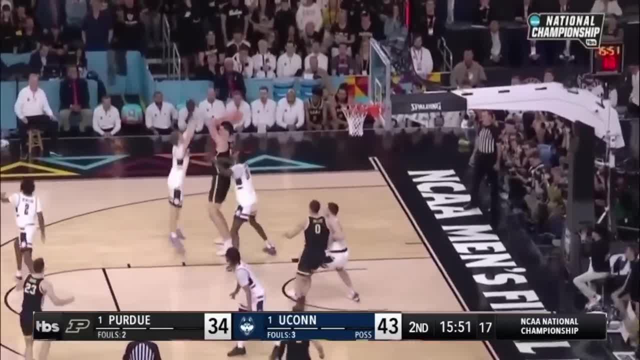 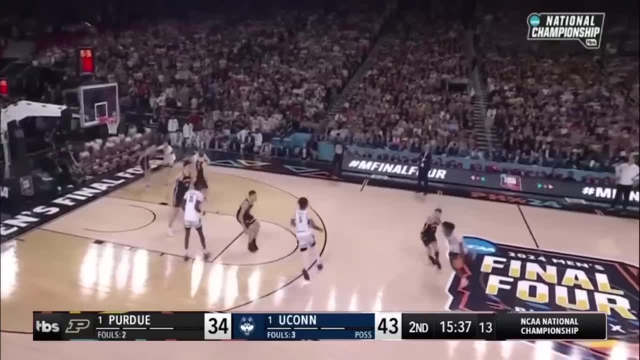 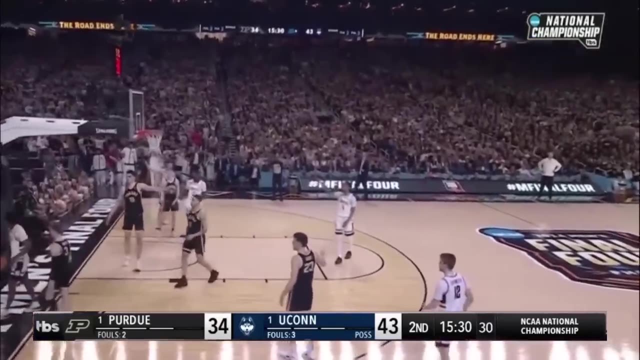 steps, Of course, open opportunities for shooters for Purdue. Johnson trying to guard, eating. they double with Spencer. It's right through the head. This is where they got to use Johnson screaming. just a zone in the back And that's what is the best. Missed it from the outside, rebound, knocked out of. we can't get the ball. 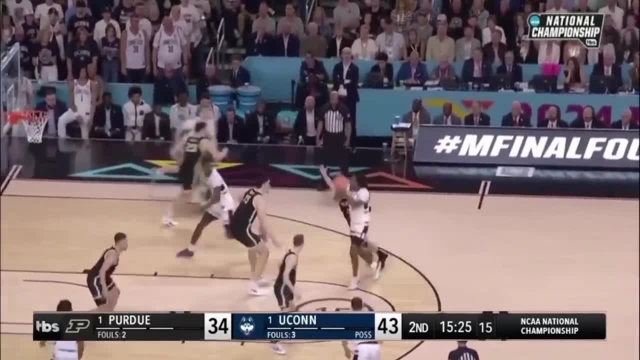 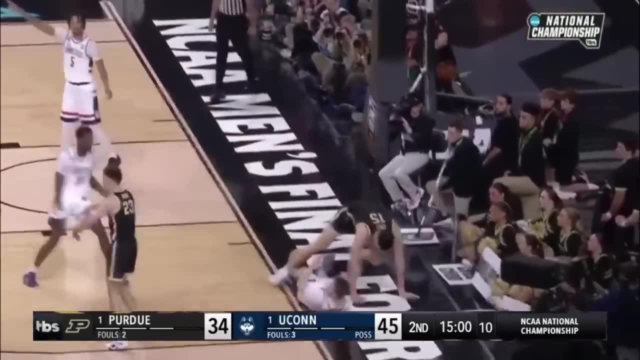 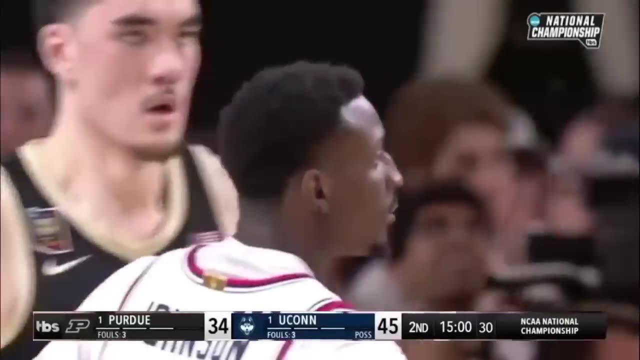 We are going to keep feeding it in to eat over and over the fouls. Instead it's gonna be the killest three way off, Spencer trying to grab it, controlled by Purdue Contact the other way they were experienced. He's gonna have make something come out a little bit. this should open up some cuts. Newton comes to the ball. 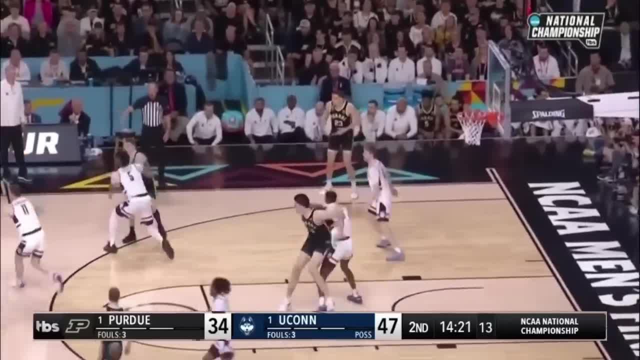 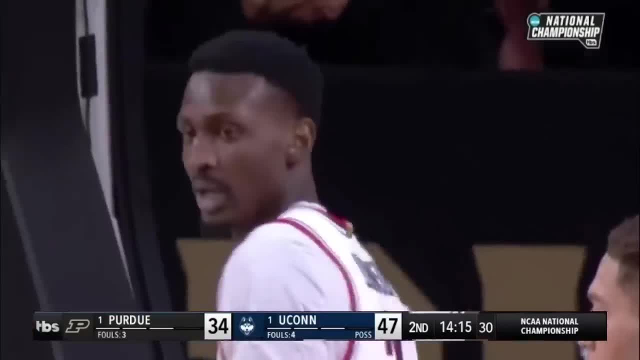 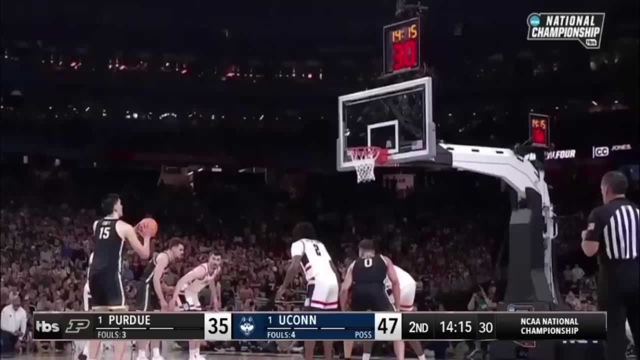 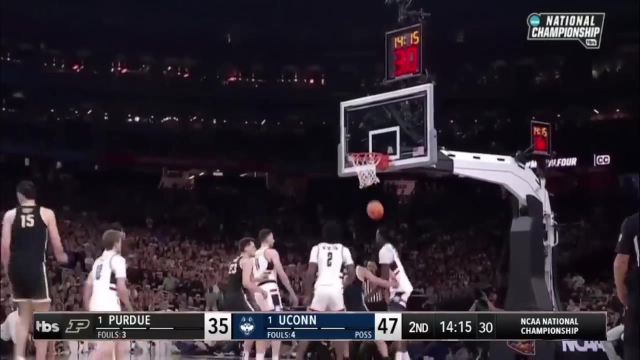 Special delivery to John, who's stuck in mud here and really solid D this trip. Edie turns By Johnson. look, three Rebounds, first player to do it in more than chance. That's what they have to do. Help Johnson out- They got somebody stepping in- or 11 minutes of game action and he cans a pair. 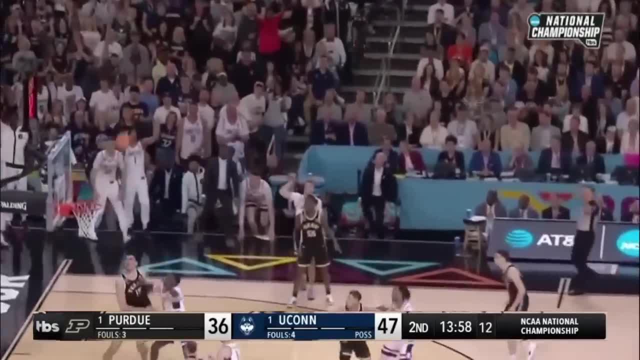 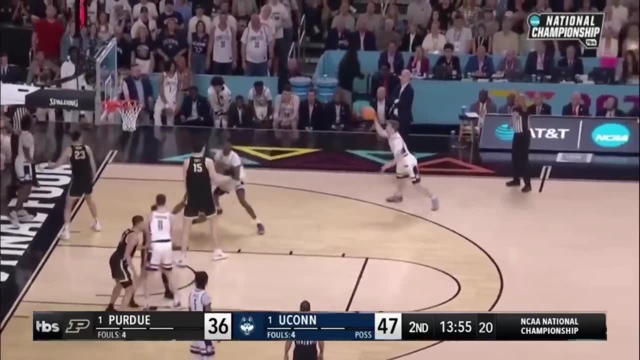 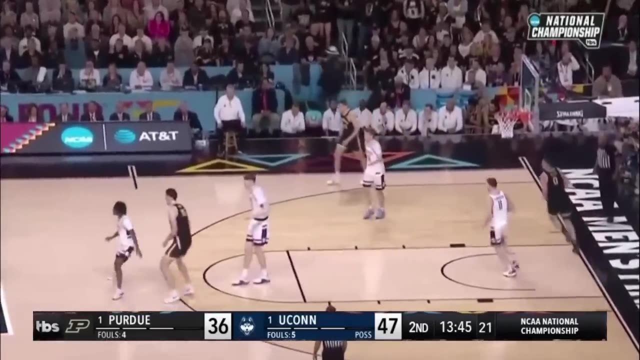 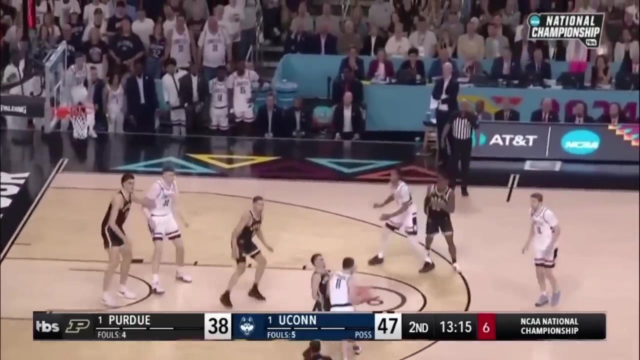 And it ricochets over to Spencer. he's gonna take it rebound. Johnson hits the deck and a problem for Edie. second fell on eating new looking triggers in. Johnson gets a moving screen. See if they play straight up now. Smith gets inside Drive and kick caravan contact- no call. Spencer penetrates and 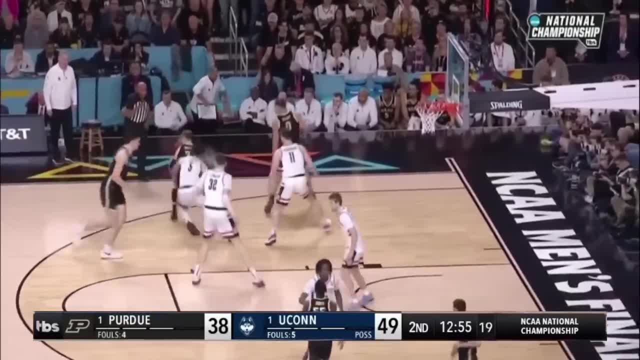 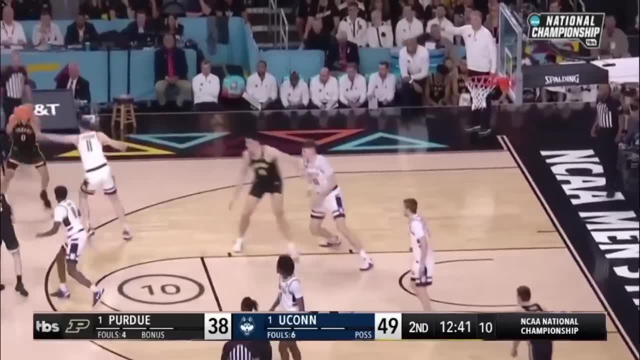 Fantastic. here on his hands, Spencer out of Davidsonville, Maryland Eadie, there's the double Spencer. they got a foul Reach in Smith. swing it. Gillis Eadie Rimming out. Oh, nice, rebound again. 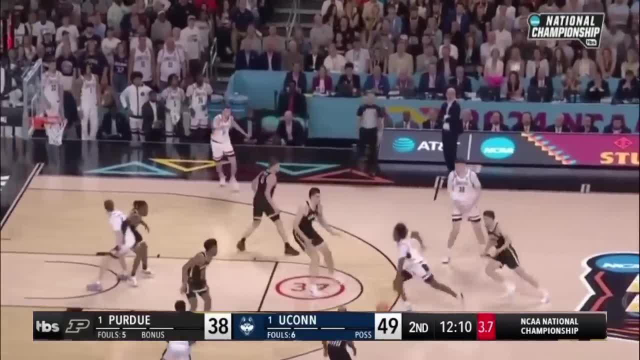 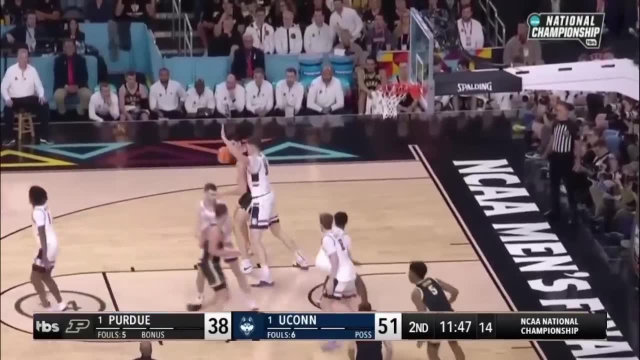 Contact from behind Mason five to shoot Newton trying to make it happen. Stop and go. Newton long stride Swips it in. He just challenged Eadie for the bucket. Right away there, Eadie double team. 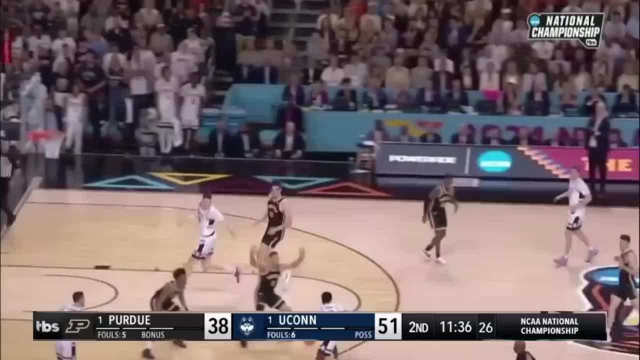 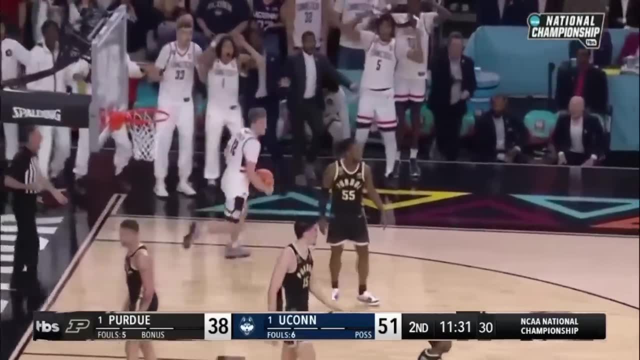 Pass it. Corner Colton Can't hit the three Good read Saturday night. they have one tonight: Caravan Short And the ball Spencer. they got a foul though. It will be Spencer, But who went to Duke? 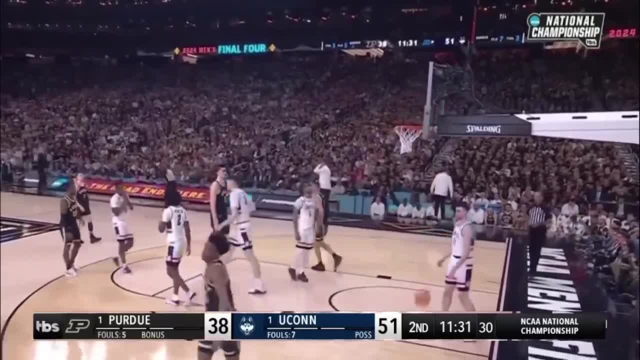 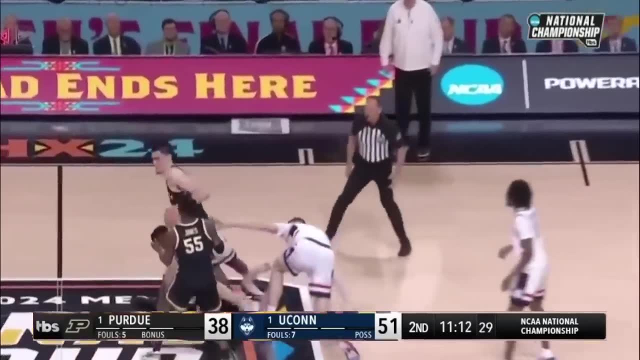 Oh, I didn't know that. Oh goodness, an air ball down. They have multiple guys who can make plays down into the clock. Smith trying to get it Dives for it. The effort by Smith and he saves it for Eadie. 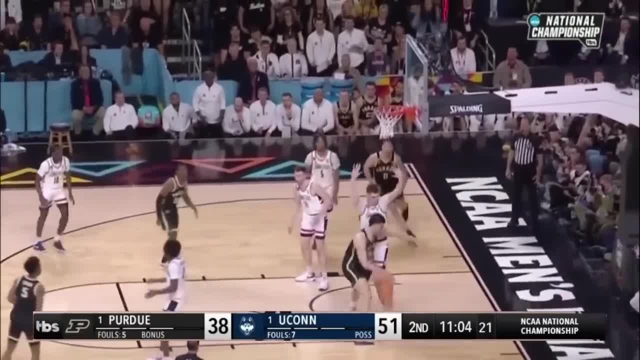 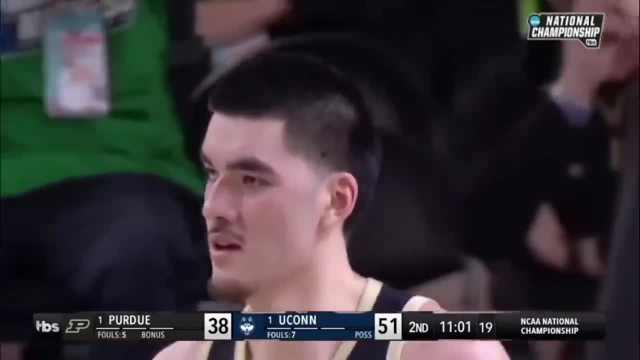 So Jones shake and bake Shows. it Bounces Eadie. Oh Well, he traveled, Not reaching down, But if we do want to get back at it, it's Castle. He just forced down a little bit. 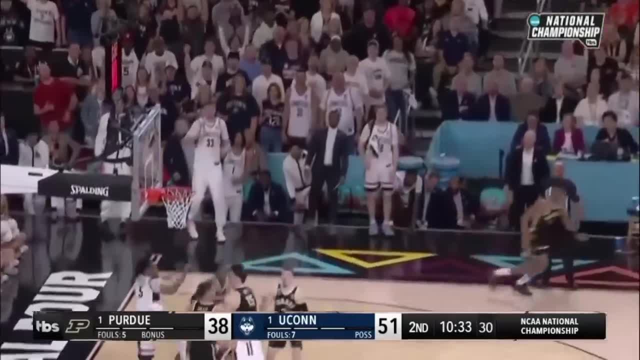 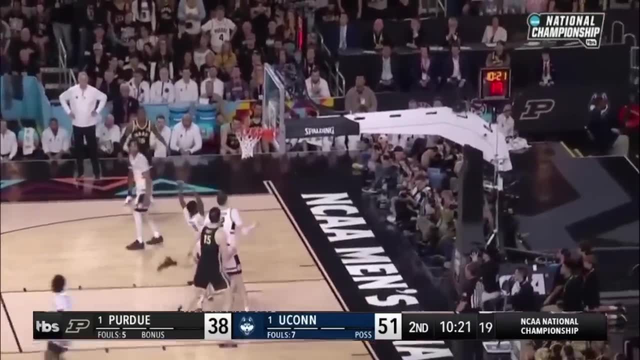 But it's tracked down by Newton Shot. clock is winding down, The jumper doesn't go to Yara, Nice rebound And Eadie engulfs it. Got to get others to light it up. besides, Eadie Smith Draws the foul on Yara. 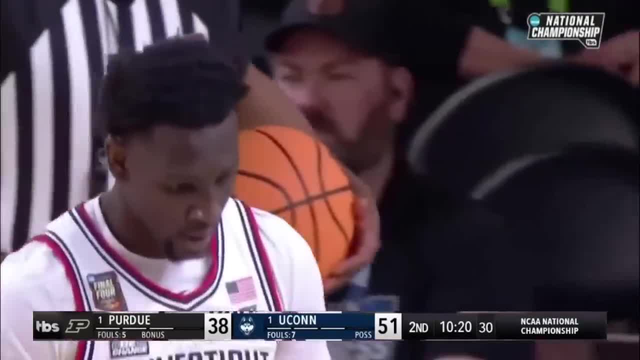 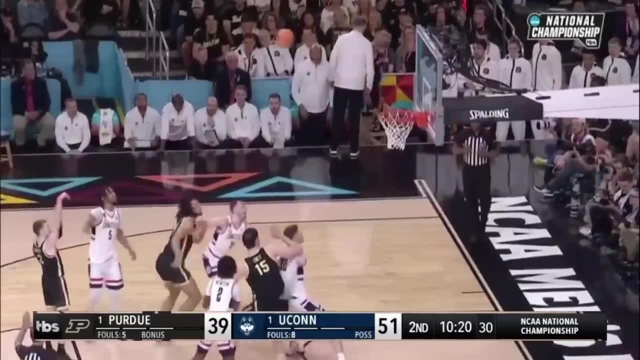 Number four, Yara, right there, but maybe this will get him going. Percent shooter, Mr Basketball in the state of Indiana. I love this kid's mind. Why'd you? He's a quintessential point guard, Mm-hmm. 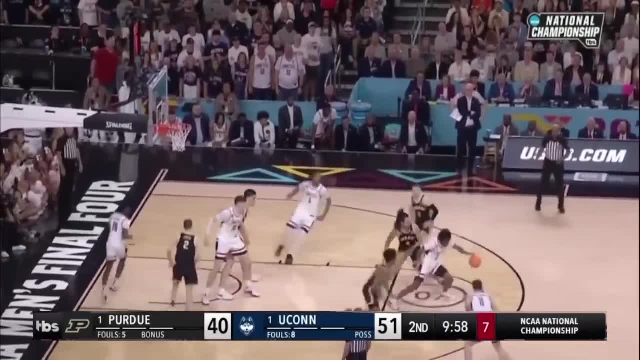 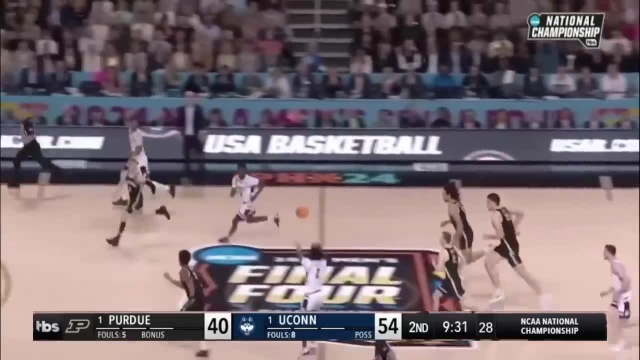 12 points, five rebounds. Spin Newton Seven to shoot Double from Colvin. It leaves Caravan open. Bingo. What a find by Newton Out of the backboard Break opportunity. Newton to Diara Right down the middle. 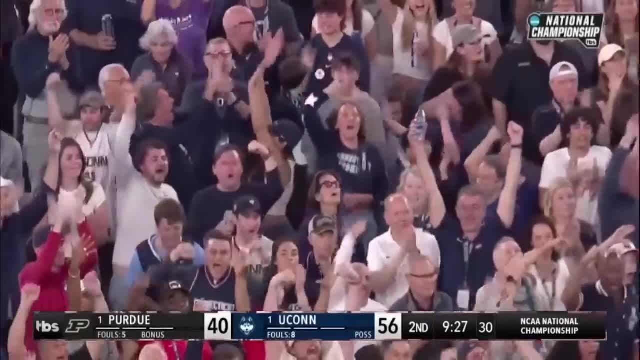 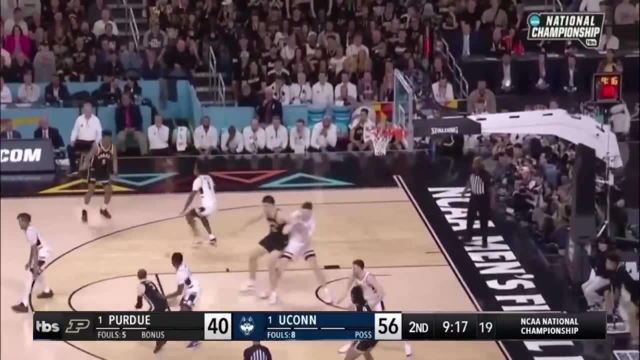 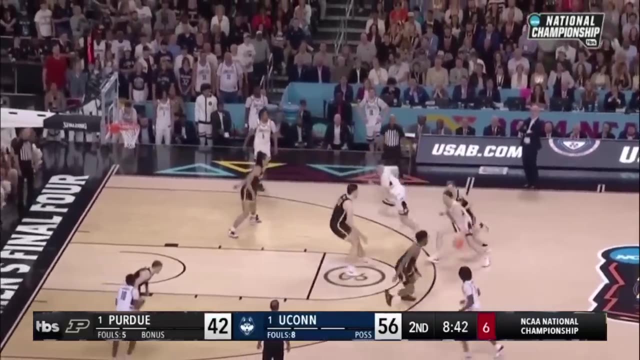 He lays it in Woo. How about that? Dan Hurley, Champion of basketball in America, Truly said: Out of the timeout, Eadie, He backs it in And they needed that. Eadie has it. Caravan using the Klingon screen. 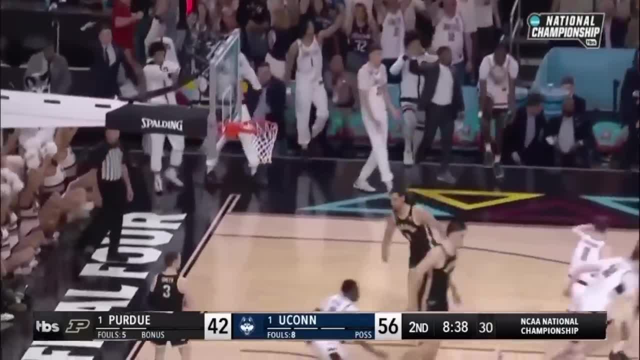 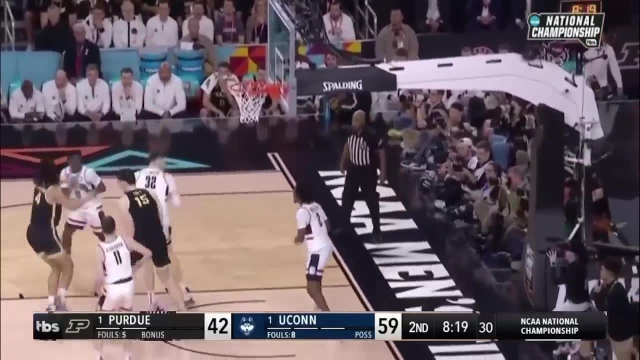 Feed it, Replace Castle Got a three. How about that? They do that. It's the same script for UConn. Really good, They could just take over the game. Smith Off the mark Klingon the board: 19 points, 10 rebounds. 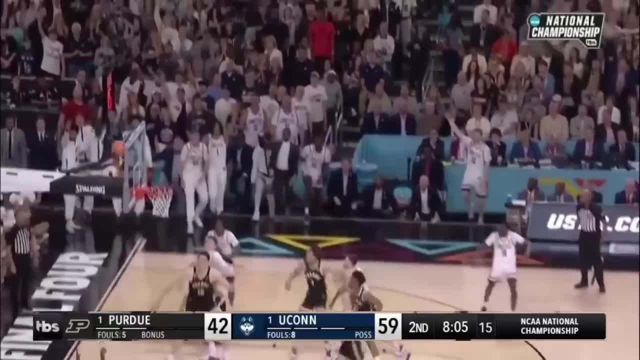 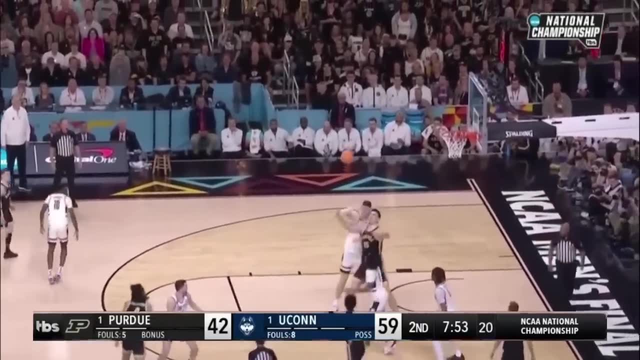 Spin it, Kicked, Caravan, Nice, Feed it Castle. Wow, In and out. Rebounded, Back it out. We are undefeated. You're eight minutes to play. They got a piece. He thought he had all ball. 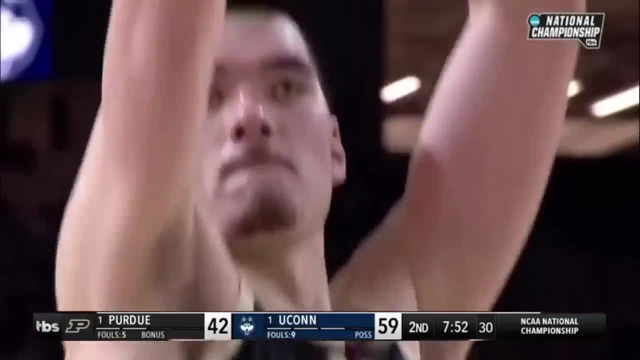 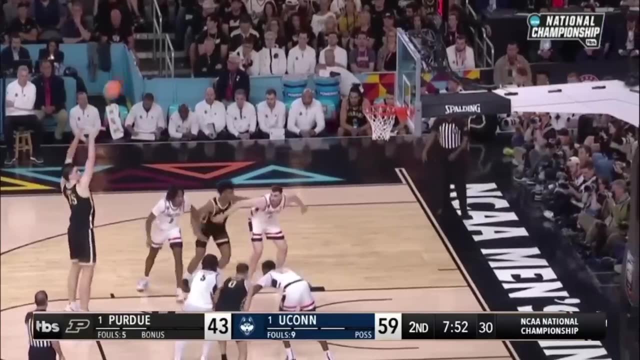 Painter, We have to indicate: Well, Dan Hurley has just coached this half. by the way, You don't need a man that led the nation in technicals. He's given a lot of credit to the timeout. The press Castle. 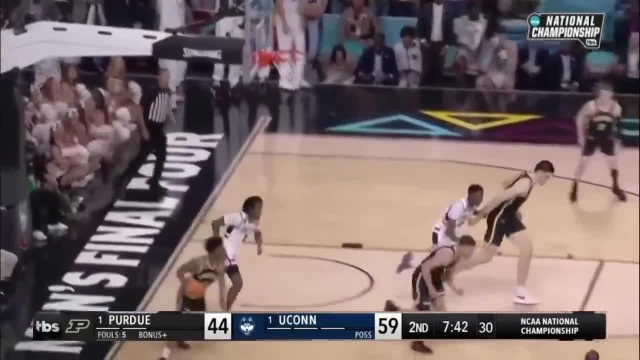 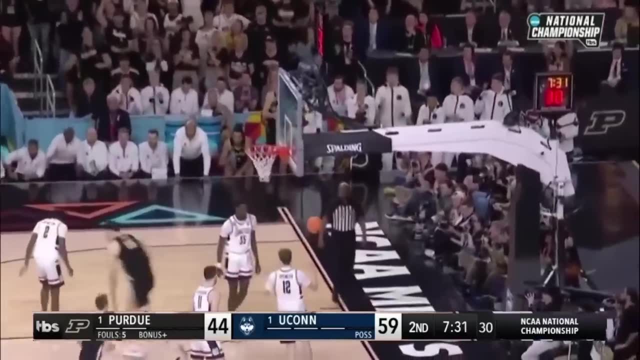 Ahead. Newton Attacks Doesn't go For Johnson And on the bench for UConn, with four fouls, Smith Feed it. He rocks the rim, But he's too big. We are going to hit the seven-minute mark of the second half. 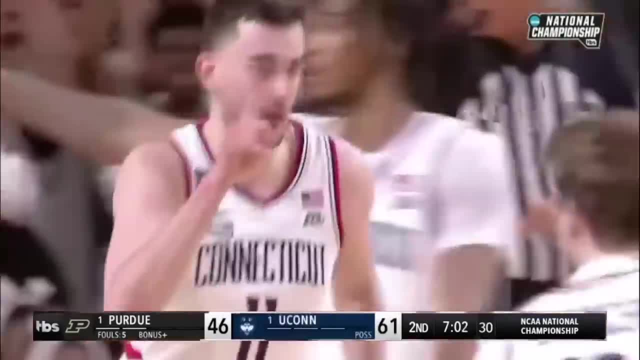 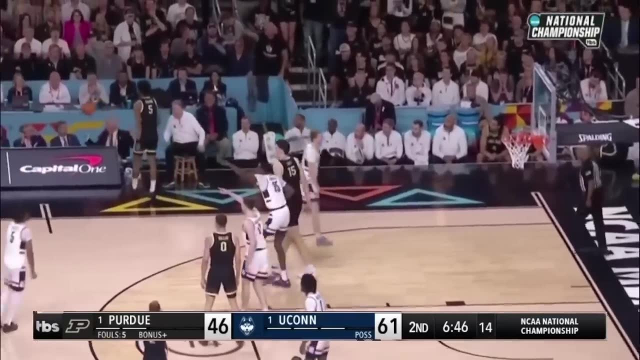 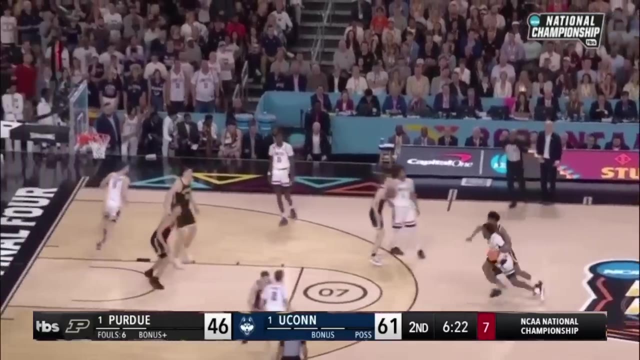 Johnson The cutter Caravan. What a slip. What a 61-46. Huskies Tip Out of bounds. Spencer creates it This summer. the target Castle at that iso on the foul lane. We've got that at a lot. 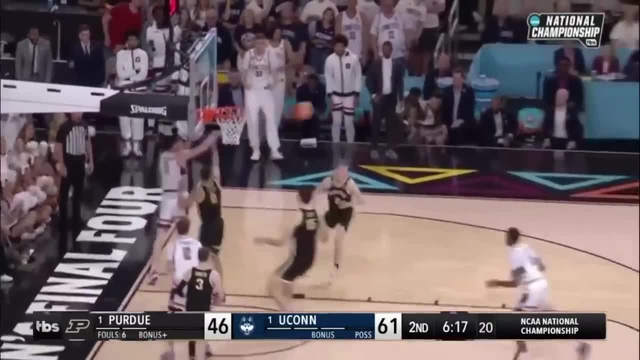 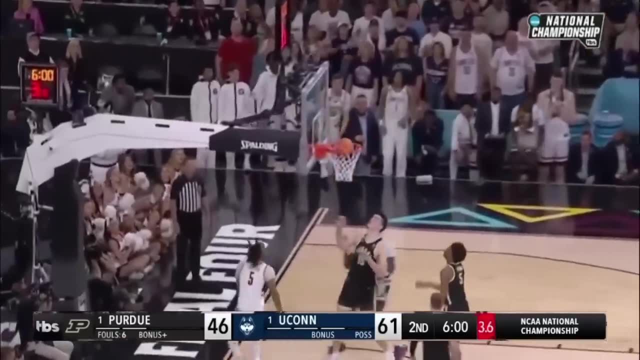 Newton, The shakeoff And the jumper doesn't go. Nice rebound Caravan Off the night. They're out-rebounding Purdue 33-24.. They grind you until you slip and fall asleep. Castle, That's clever Nature. 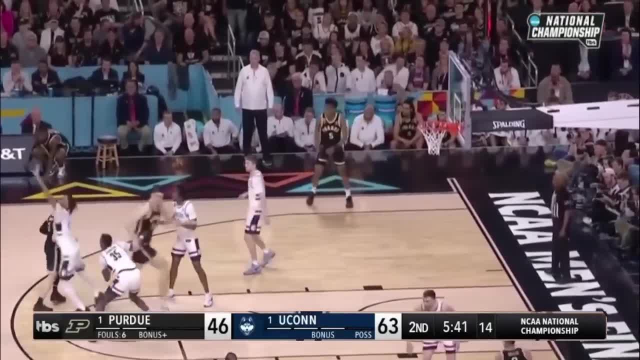 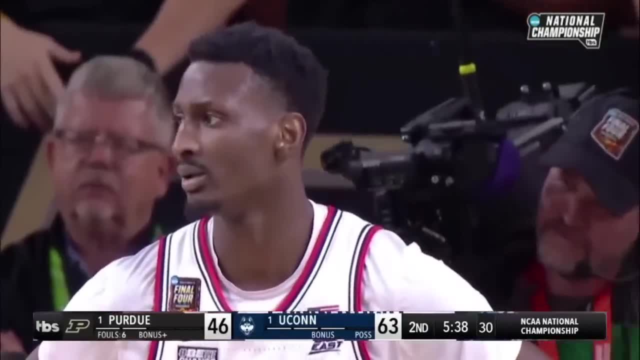 Dan Hurley. This team possesses Way outside Eady To Lawyer. They need buckets, Doesn't go And they get it on. There was a crowd there on the interior: Johnson, Sign up for this. He's going to be defending the big fella. 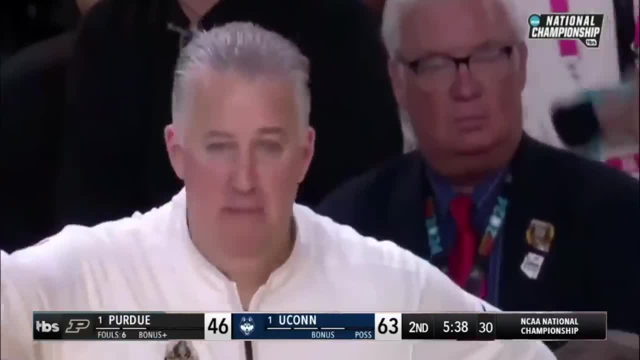 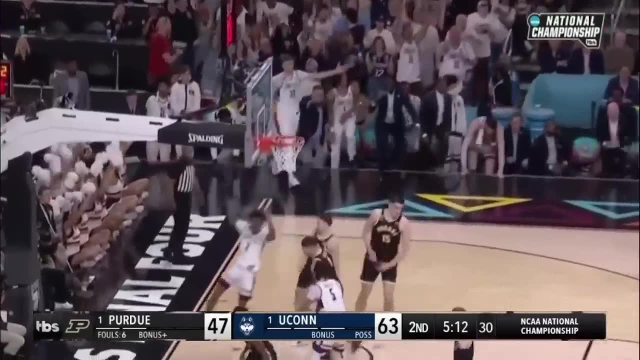 The floor. We'll just own up, though, I think, Don't you? Yeah, Not Eady on Diarra. There it is again. Spencer Stops Pops. Yes, sir, Wow, He's got some stuff, Spencer. 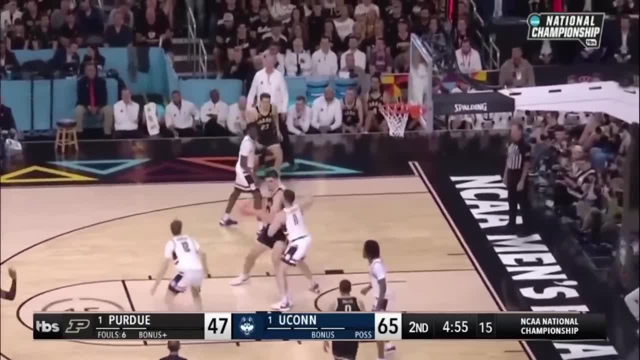 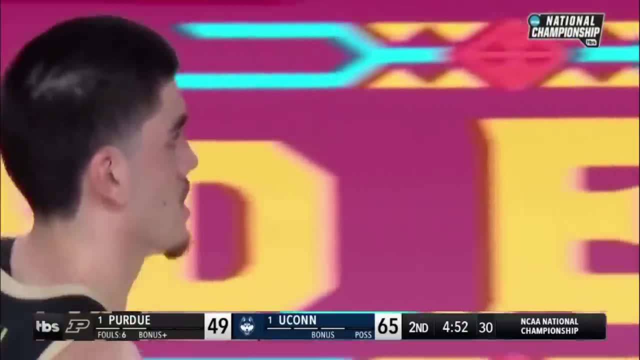 Look at him. He's fighting him. Caravan Eady- Ooh, He's using the muscle Caravan actually now has 29.. He's going to need a facial for Byron. He's been running four points And Smith has chipped in with 11.. 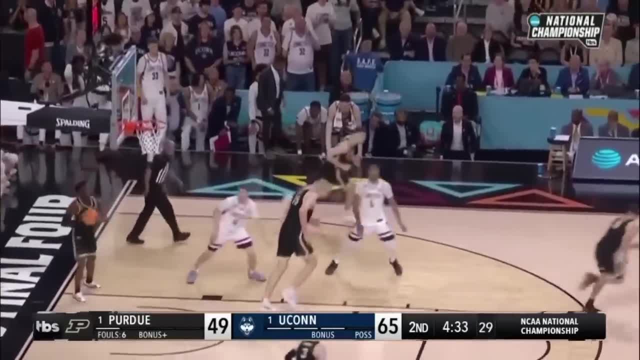 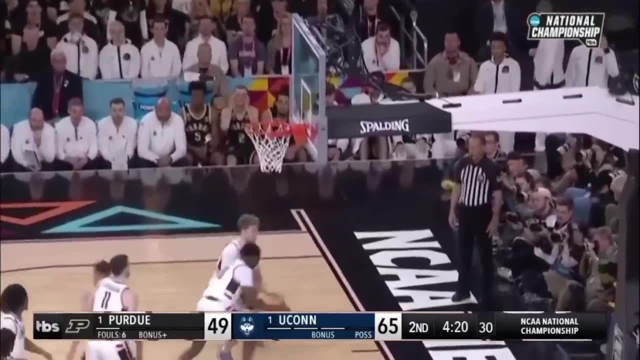 There's no easy out. Caravan takes a look. He didn't need that right there That early in the. Heidi Feeds it, Eady Missed it. Riebe Drop defense, Newton fend off. 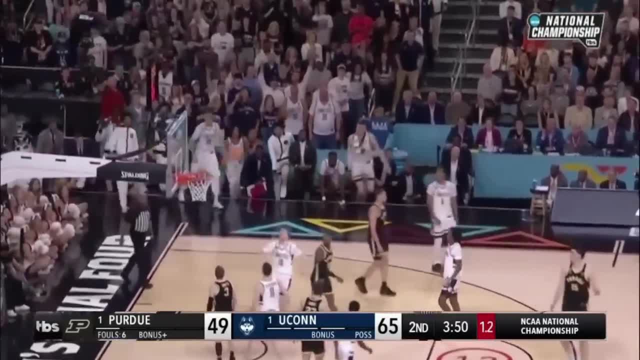 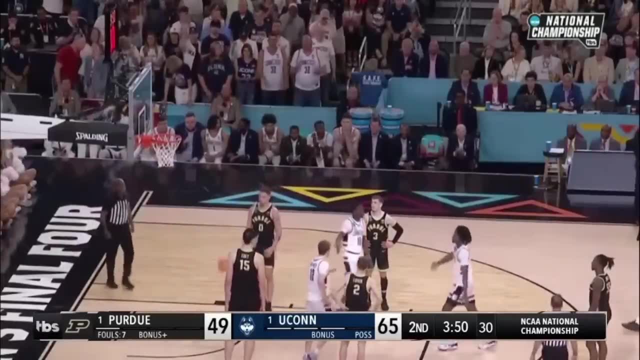 Shot clock down to three Newton steps in and draws the foul on Eady Team effort which Dan Hurley has preached to his. Of course, Geno had a great run too, wherever this year Lost in the 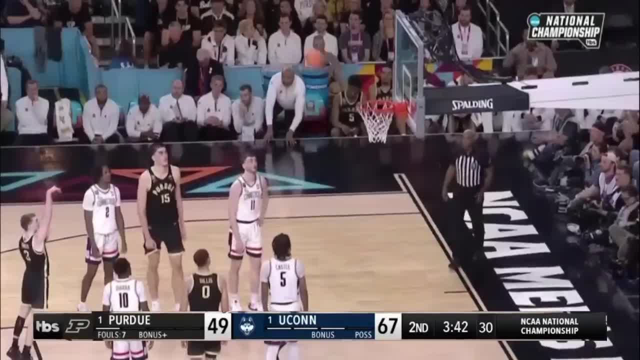 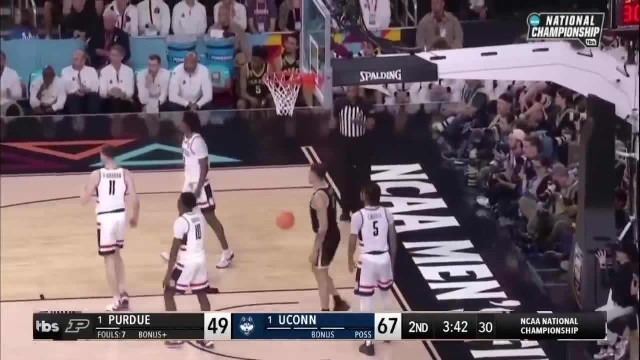 It just doesn't happen often. Well, it's been. incredible Principles, The same focus and determination, The determination that Dan Hurley is really emphasizing Friends to catch up with his defense. And what I loved when he talked to us yesterday was how he 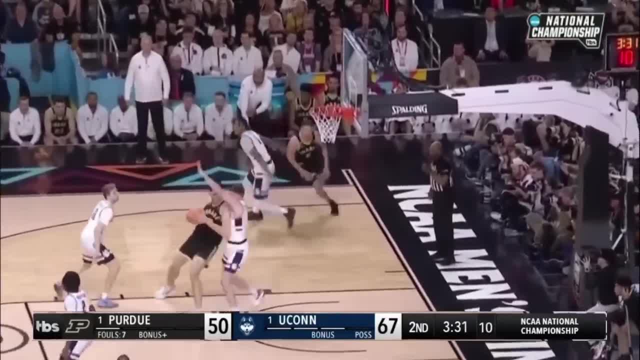 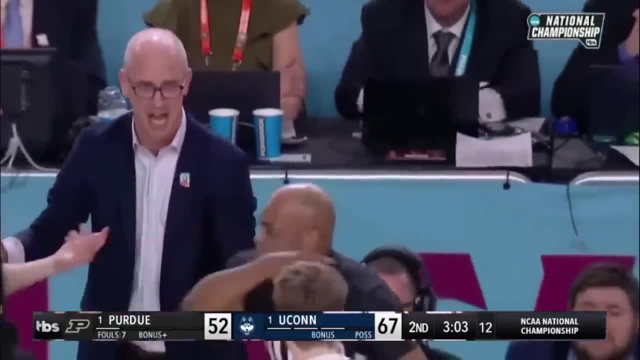 Jones feed it to Gillis. They're going to stay at home. Caravan Eady steps in for two Caravan may have to go to the Communicate with Cam Spencer. It is good appreciating though Eady on a kick. 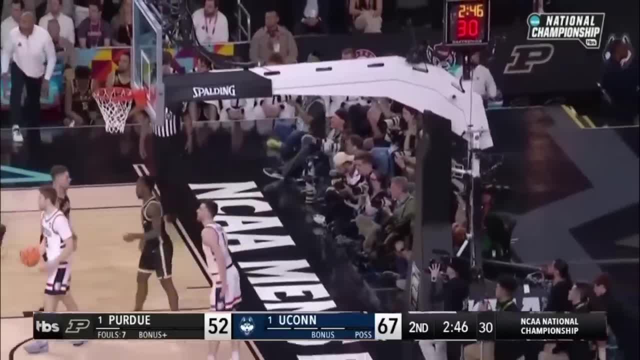 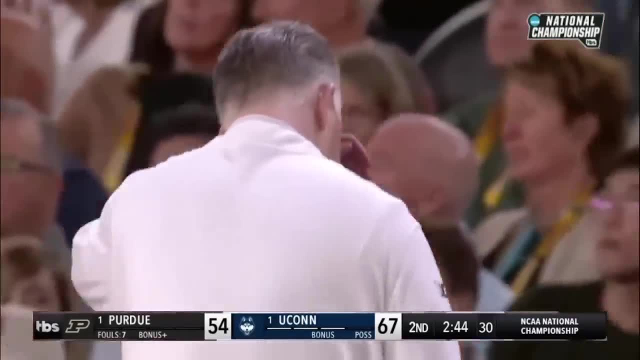 Jones penetrates, Leavitt Gets the roll on the inside Timeout. Get by his people as well. Thirteen point: Had a great trap We did. Lance Jones rotated there The national championship game And right now they're in a big hole. 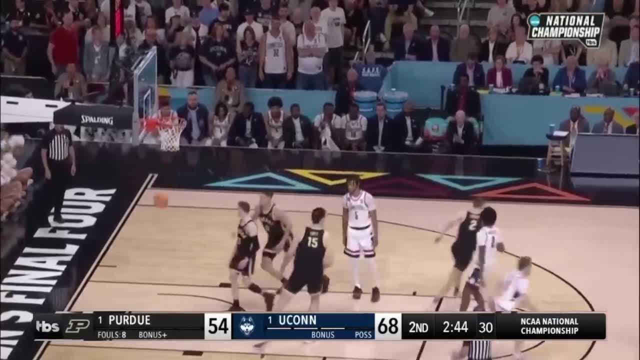 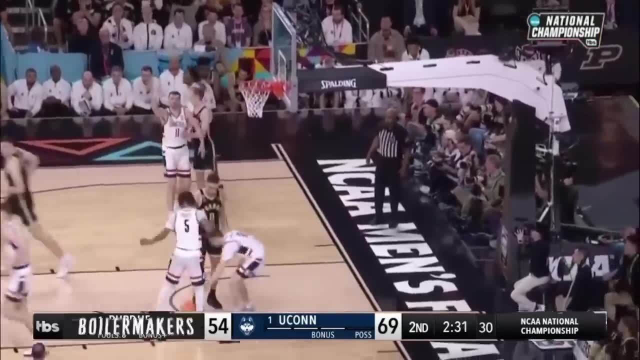 They are, But we All of them put themselves in position, The only additions. Lance Jones of, In effect, On this roster from the state of Indiana. He is not one of them as he puts it down hard against Klingon. 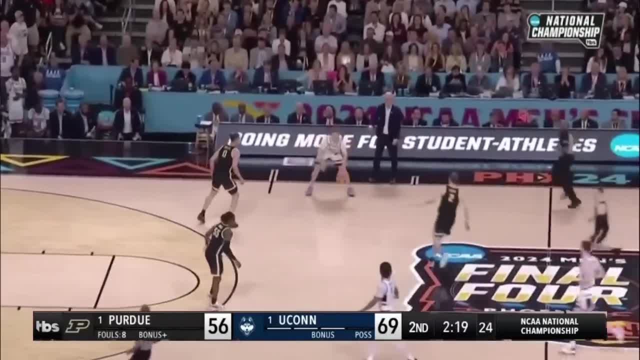 And Klingon couldn't do anything for foul. He'd go out of state for somebody like that. Yeah, I think so. There's high school here in the states. He played at IMG Academy, but he was a backup. He was not. 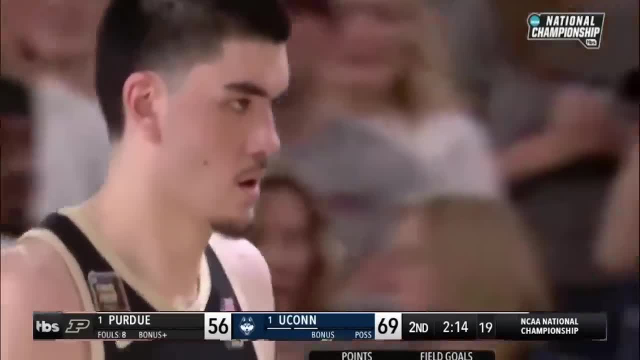 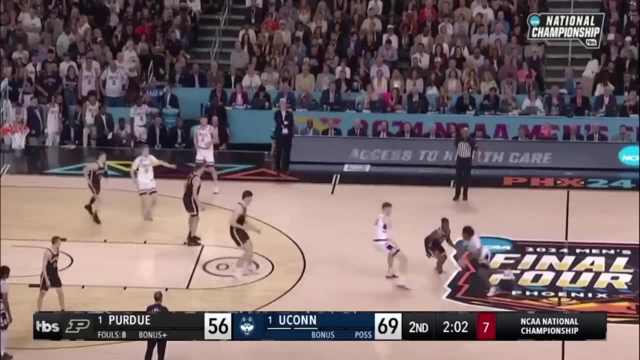 And right there, Cam Spencer calling a timeout, But went to the corner To call it For him On their roster in the NBA. I mean his improvement. While doing it, Screen Klingon Caravan takes the big snap.